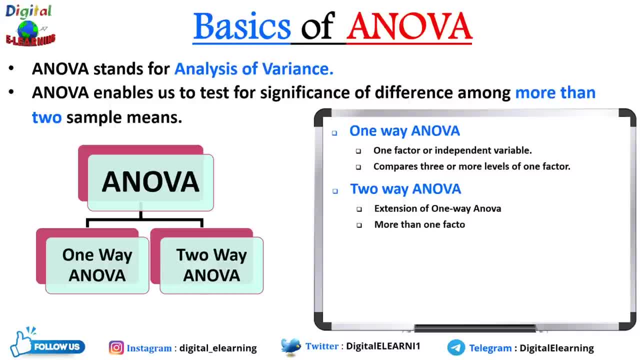 about. it is basically an extension of one-way ANOVA and more than one factor or independent variable is there. It compares the effect of multiple levels of two factors and the test statistics in ANOVA. So now we look at some assumptions for ANOVA. The population from where the sample is drawn. 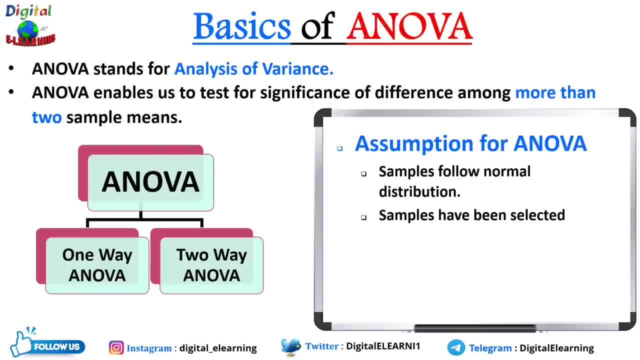 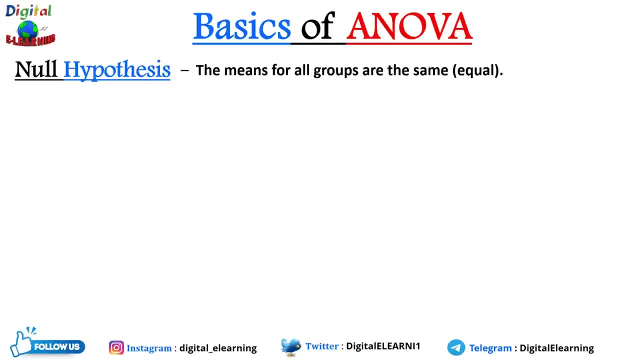 should follow a normal distribution. The samples have been selected randomly and independently. Each group should have a common variance and data are independent. These are some of the assumptions while we work on ANOVA. Null hypothesis for ANOVA says The mean for all the groups are same or equal. So H0., That is, mu1 is equal to mu2 is equal. 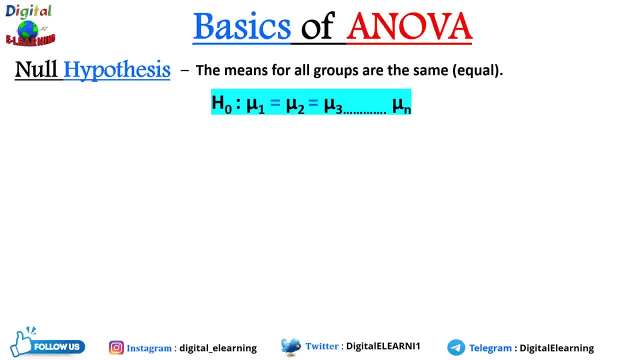 to mu3, so on up to mun. And mu denotes the mean. An alternate hypothesis would be that the mean are different for at least one group of pair. So H1- that is alternate hypothesis- denotes mu1 is not equal to mu2 is not equal. 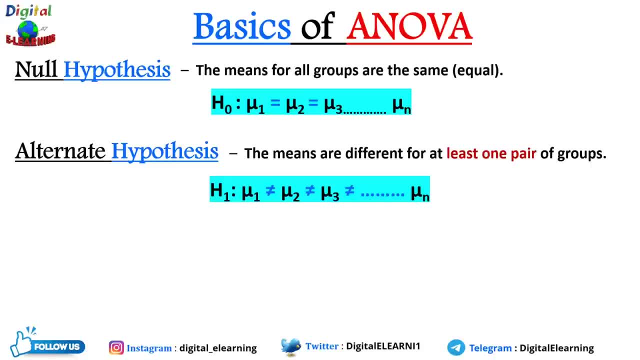 to mu3, so on up to mun. If any of the group mean is significantly different From overall mean, Then the null hypothesis is rejected. But here we are comparing more than two means. But if you only want to compare two groups of mean is use the t test here. 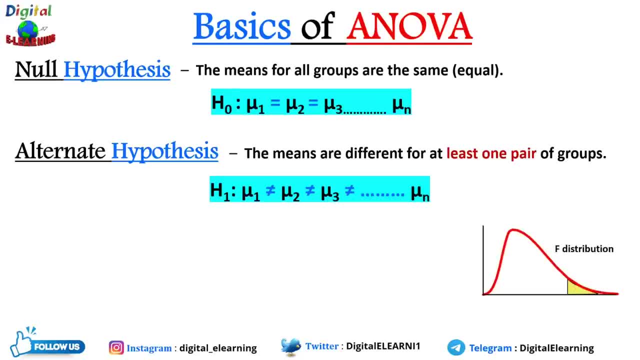 ANOVA uses the F test for statistical significance. The F test comprises the variance in each group mean from overall group variance, That is, variance between divided by variance within. So if the variance within, So if the variance within The F test will find a higher F value, Therefore likelihood that the difference observed is. 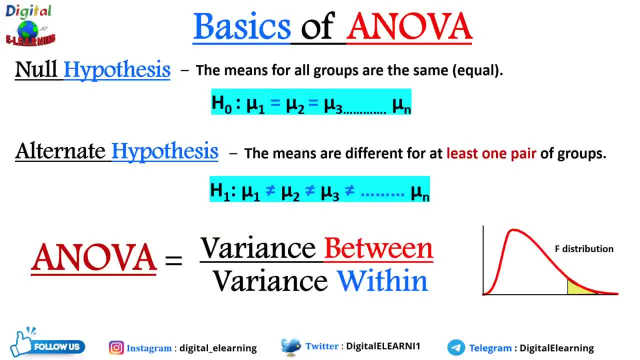 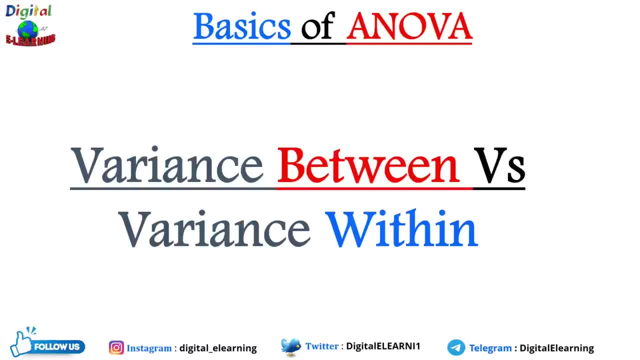 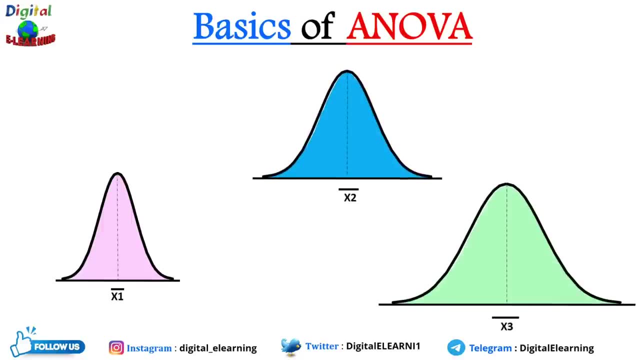 real and not due to chance. Now let us see what's the difference between: variance between and variance within. Suppose you want to compare three sample means- X1,, X2, and X3- to see if there is any difference exist among them. Yeah, 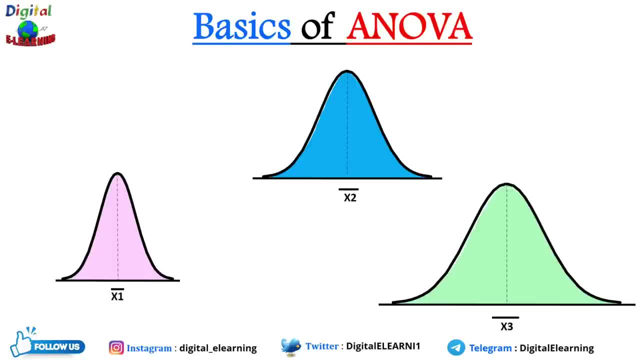 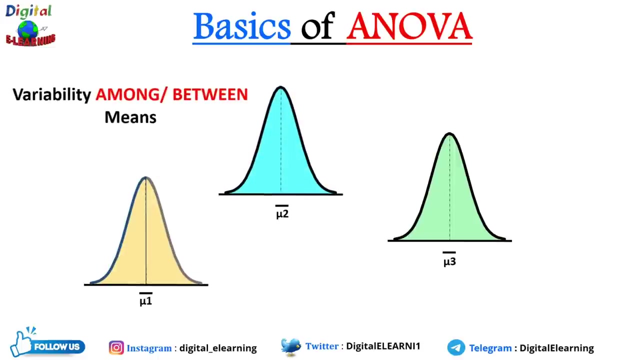 So question here is whether they all are coming from same population or not, or one mean is slightly offset from other two. So variance around or variance within distribution is an internal spread or variation of each distribution like this. That is variance within or variance around. We'll take again the three means: me 1, mu 2, me 3 and plotted for: 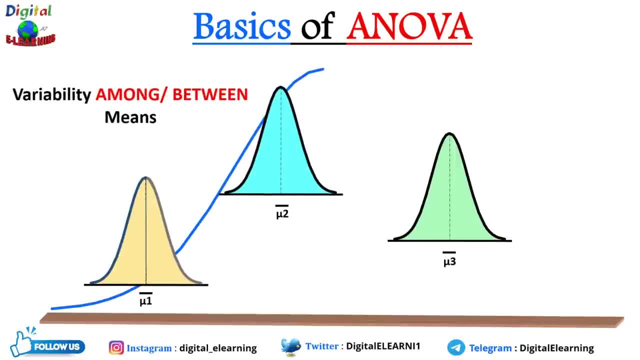 Variability among and between plot and under normal curve to see what is the distance of each mean from the overall mean here. so in this case a null hypothesis would be: mu 1 is equal to mu 2 is equal to mu 3 and Alternate would be: either mu 1 is not equal to mu 2 or not equal to mu 3. 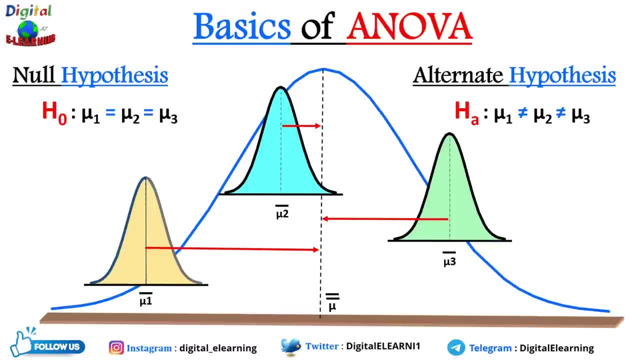 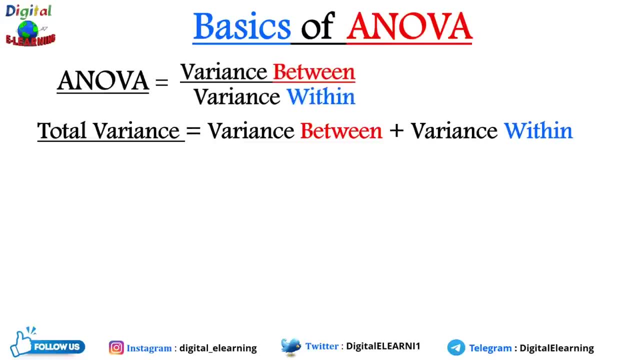 That is how we calculate variance among and between. here, ANOVA is basically a ratio of variance between divided by variance within. a total variance is the sum of variance between plus variance within. if Variance between by variance within ratio is greater than equal to 1, we reject the null hypothesis. 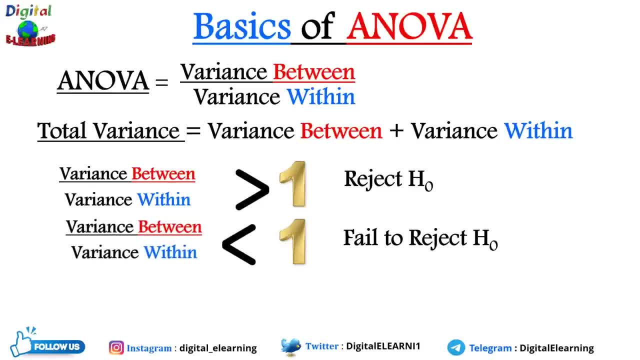 If it is less than 1, we fail to reject null hypothesis. if it is equal to 1, again We fail to reject the null hypothesis. So what does this state? that is, if the between group variation is high Relative to within group variation, then the F statistics of ANOVA will be higher. 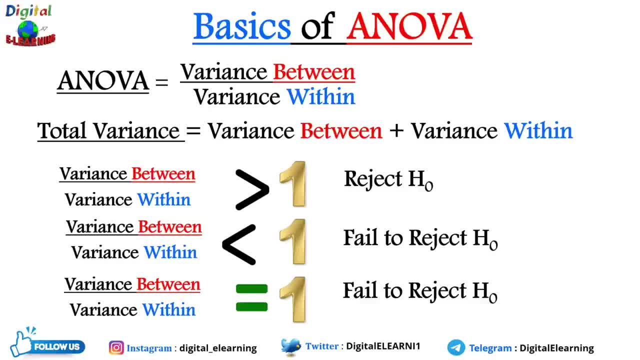 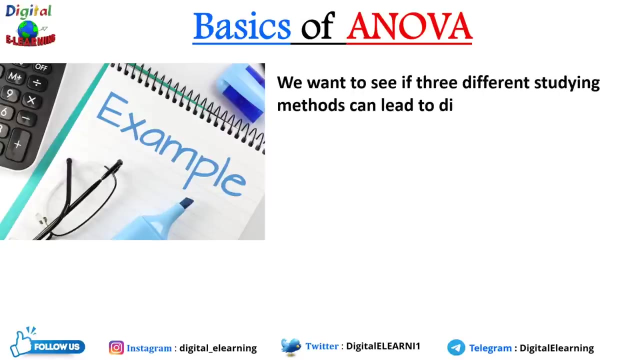 And the corresponding P value will be lower, which makes it more likely that we reject the null hypothesis that the group mean are equal. the larger F statistics, the greater the variation between the group means relative to the variation within the groups. Let's take an example. We want to see if three different study methods can lead to different mean exam scores or not to test this. 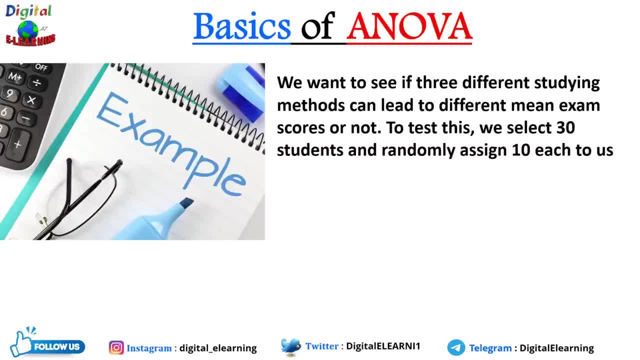 We will select 30 students and random. We assign then each to use a different studying method. We solve this example using two different methods. Let's look at method number one. This case will use the method one. So this is a data. we have method a, b and C. 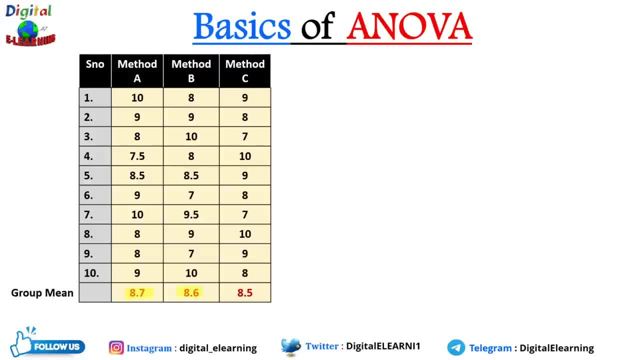 this is our group mean at the bottom: eight point seven, eight point six and eight point five for method a, B and C respectively, and all, all mean is the average of eight point seven, eight point six, eight point five, which comes to eight point six. now will first, will create the 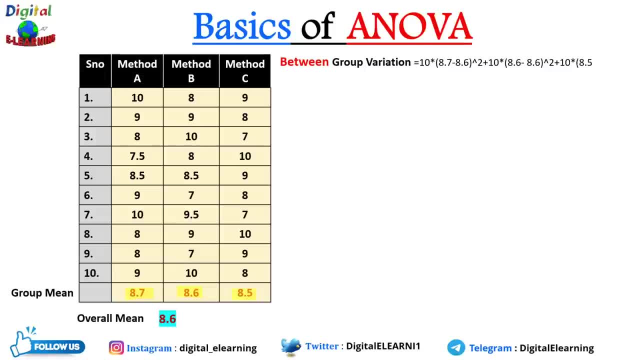 the between group variation which is like 10, which is the total number of quantity 4 into 8.7, that is the group mean of a minus 8.6, the overall mean square. then for group method b will have 10 into 8.6, minus 8.6 square, plus 10 into 8.5, the group mean from c minus the overall. 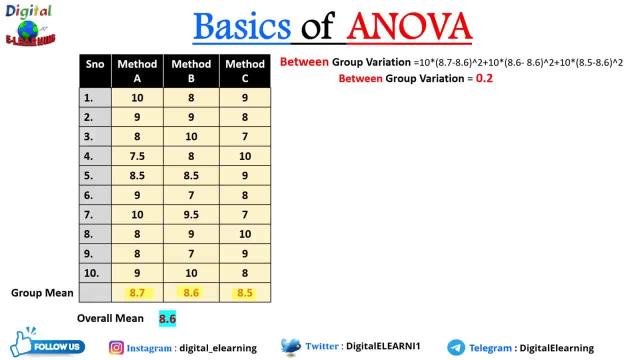 mean square. this is where we get between group variation as 0.2. now we need to calculate within group variation. that is, summation of x ij minus x j square, where x- no summation, x ij is the ith observation in the jth group and xi is the mean of j group. so method a we will create within group. 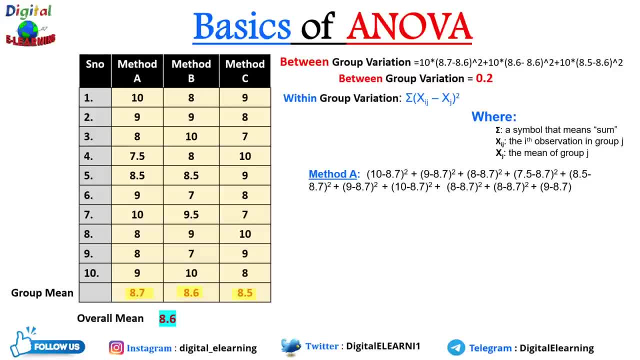 variation. so that is 10 minus 8.7. 8.7 is the group mean of method a square. now we will subtract each value from their group mean to 10 minus 8.7. square plus 9 of 8.7 is the group mean of method a square. now we will subtract each value from their group mean. 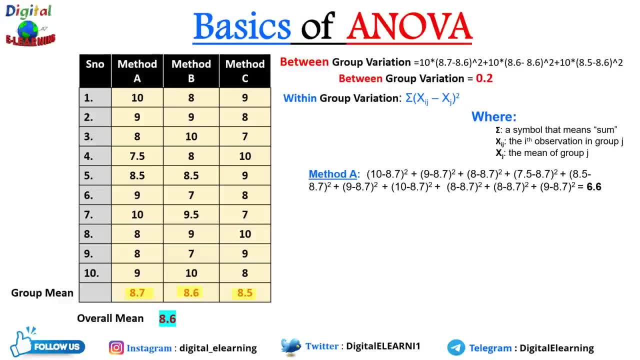 minus 8.7, square plus 8, so on, we'll get for all the values for 10 and it comes to 6.6. similarly, we will do it for method b and method c as well. now we need to sum this: all values which which we have received for method a, b and c, that is your total group variation: 6.6, 10.9 and. 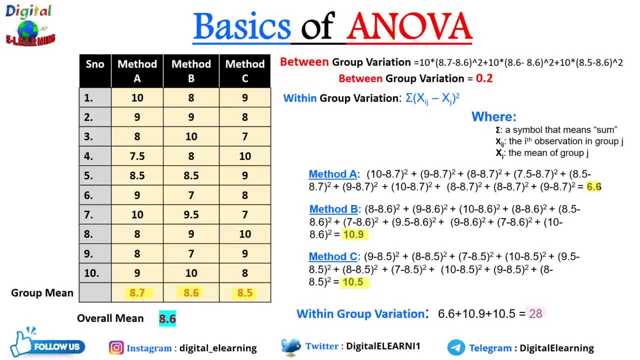 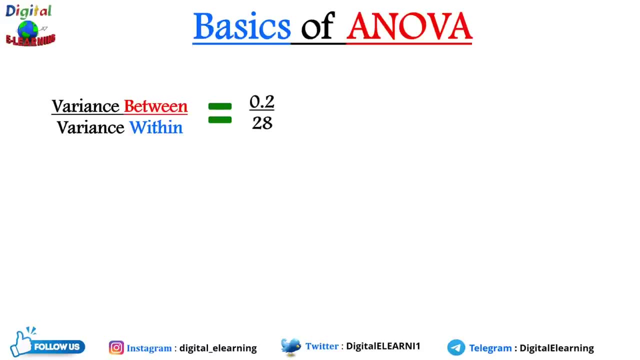 10.5, which comes to 28. now you remember these two values: between, group variation was 0.2 and within, group variation is coming as 28. now we'll put these values in this formula: variance between and variance within. so we get 0.2 divided by 28, which is 0.0071, which is less than 1. so we fail to reject the null hypothesis. 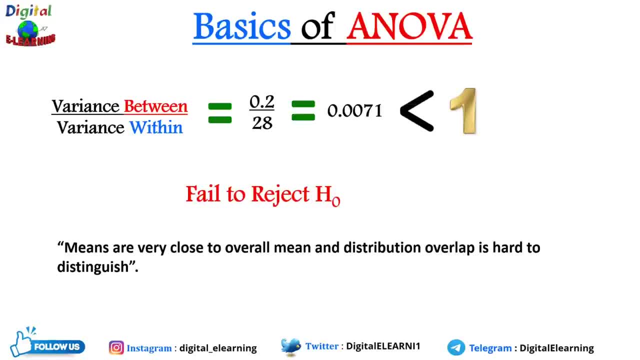 as per the initial assessment, that is, mean are very close to overall mean and the distribution overlap is hard to distinguish. that is the analysis that we have now. we'll use the second method and we'll use the second method, and we'll use the second method and we'll use the second. 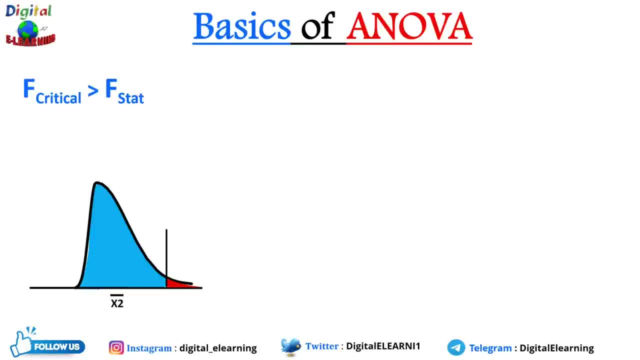 method using f table. so in this case, if my f critical is greater than f stats, we fail to reject the null hypothesis. if f critical is less than f stats, we reject the null hypothesis. in our case, assuming that alpha or level of significance is 0.05, we will quit f stats, which is like: 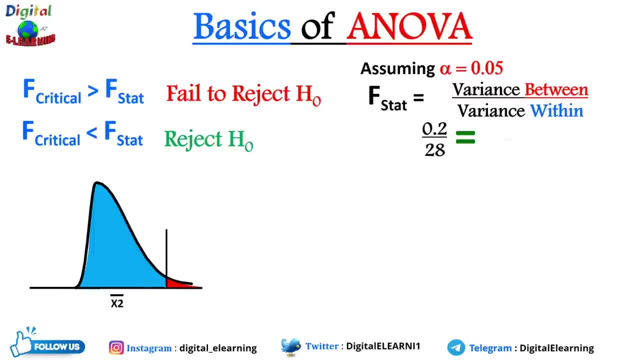 variance between, by variance within which is like what we have calculated, which comes to 0.0071 f critical value, which is here, after which everything we have to reject the null hypothesis. so, and if it falls in this region, we fail to reject f. critical is the numerator degree of 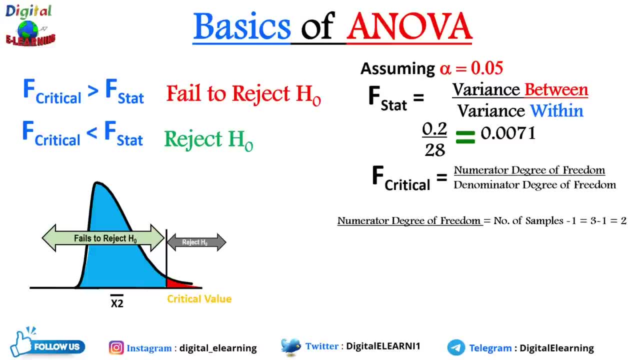 freedom divided by denominator degree of freedom, and we have to look into the f table, but before that the numerator degree of freedom is number of samples minus one, so number of samples where we have three. so three minus one is two and denominator degree of freedom is the total. 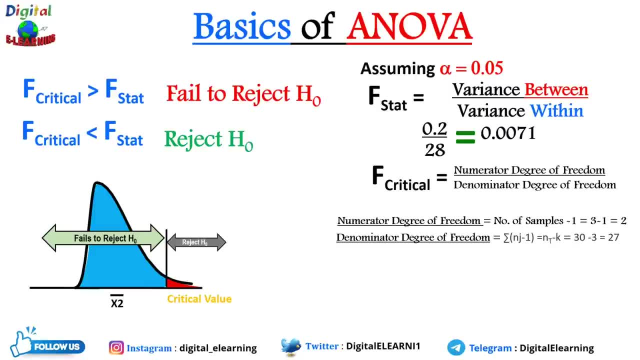 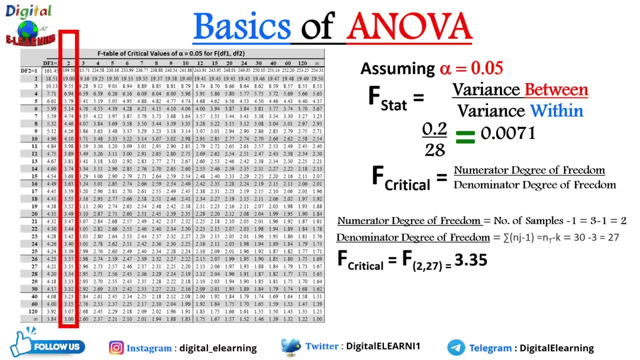 number of values minus three and which comes like thirty minus three is 27. we look at this value of f2 and 27 critical value from table. we'll look at how we get three point three, five. so this is a numerator degree of freedom and this is the denominator degree of freedom and we get a common 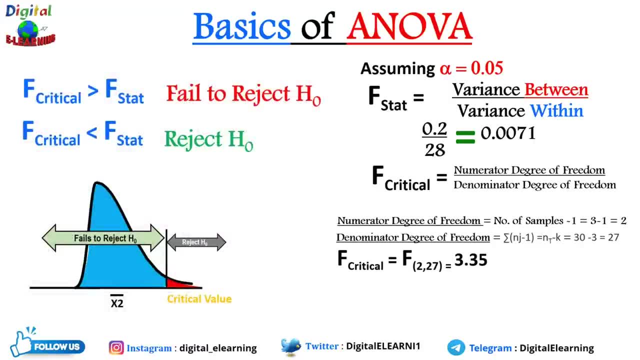 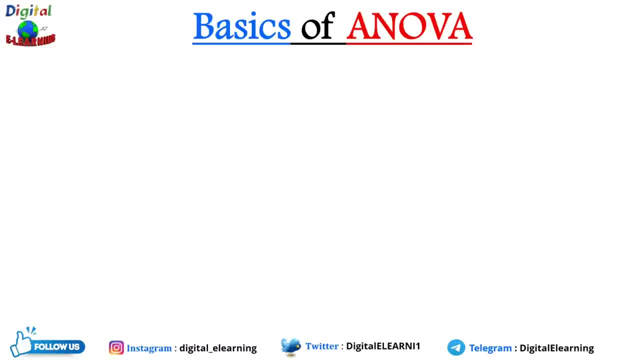 value as three point three five at intersection. so that is why in our case f critical, that is, three point three five, is greater than f stat, that is 0.0071. so we fail to reject the null hypothesis here. so let's understand the all the sources of variation here. so we have total variation sst. 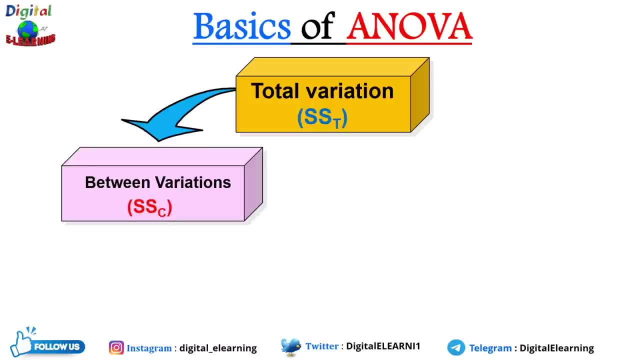 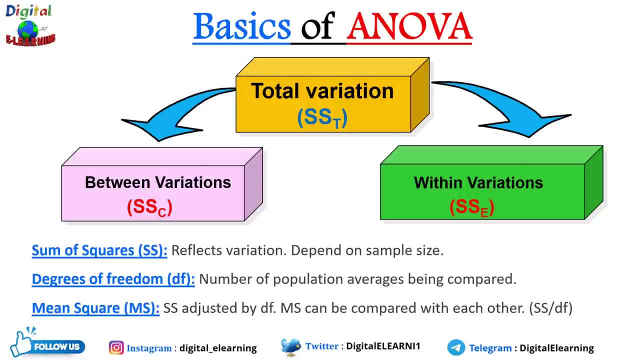 which is further bifurcated into between variation, which is ssc, and within variation. sse and ss denotes the sum of square which reflects the variation and depends on sample size. degree of freedom is the number of populations average being compared, and mean sum of square, ms, is the ss. 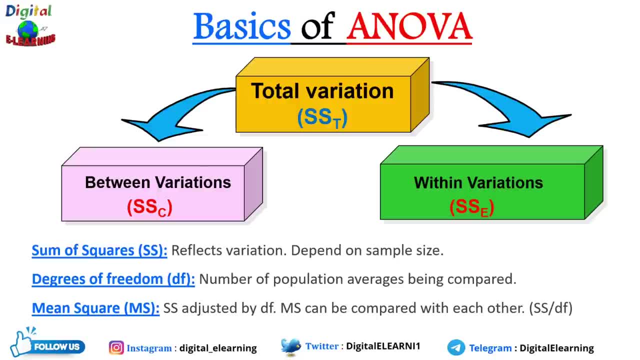 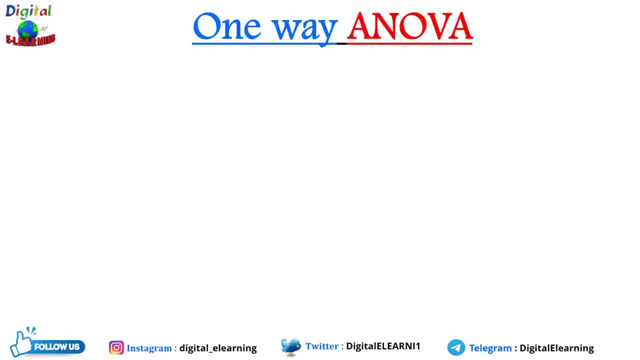 adjusted by degree of freedom, so ms can be compared with each other like the sum of square degree of freedom. so ANOVA involves calculation and interpretation of number of parameters which are summarized in this table. this is a typical one-way ANOVA table, so the row one relates to 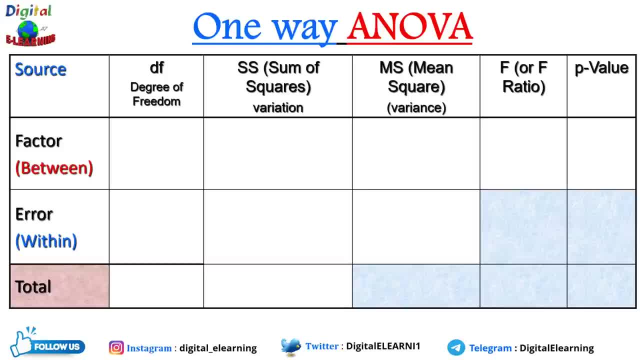 variation between the mean of the group. the values are almost always either referred to as between group or are identified by grouping factors. the row two refers to variation within each group, meaning the sample standard deviation for each group as compared to the number of variables, and the row three refers to overall performance of the other group members. and the row three 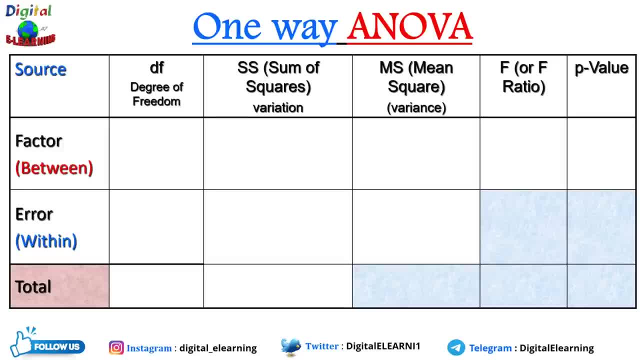 refers to total variation. under the column section of ANOVA table we have following subjects like sum of squares, degree of freedom, mean square, f ratio and p value. so for degree of freedom they are different groups. therefore a minus one is the first degree of freedom for between group effects. 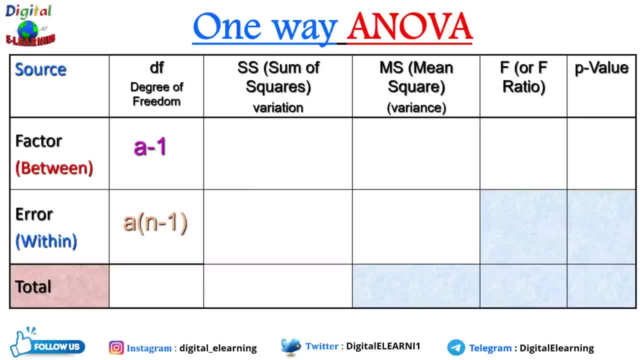 and for degree of freedom. for within group it is equal to a into n minus one. right for, and total would be if you add both these. for sum of square, this is the term which are calculated by adding the series of square error terms. so for between variation, it is SSB. 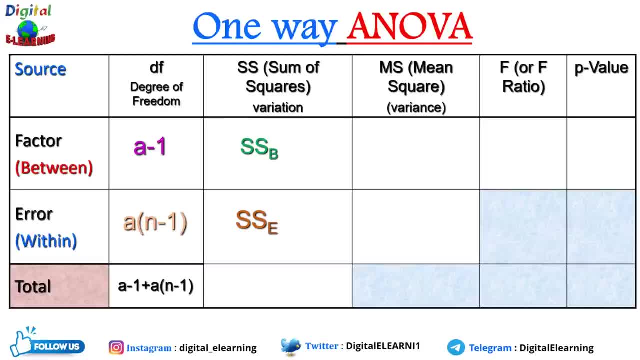 for error. it is SSE that is within variation and total would be if you add both. these two mean square are the key terms in classical ANOVA. it is calculated by mean square between, for between variables, like SSB divided by degree of freedom, a minus one. similarly for MSE would be SSE divided. 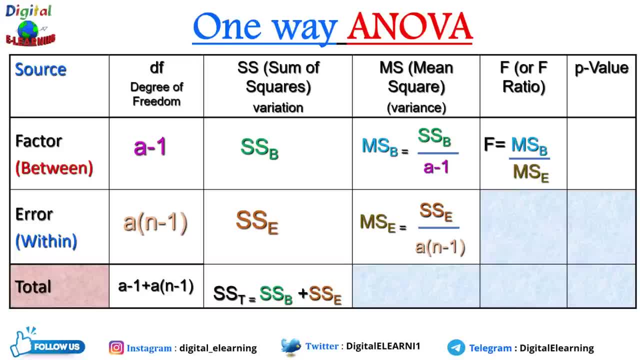 by a into n minus one, and then f ratio would be the ratio of Ms between variation, but by Ms error or within variation, and correspondingly we will calculate the p value. so if all the mean are equal, the two mean square should also be not significantly different. 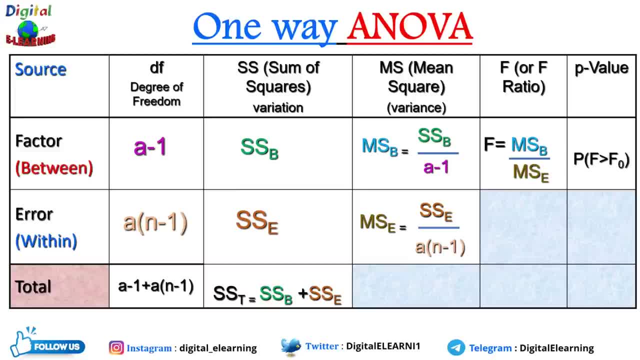 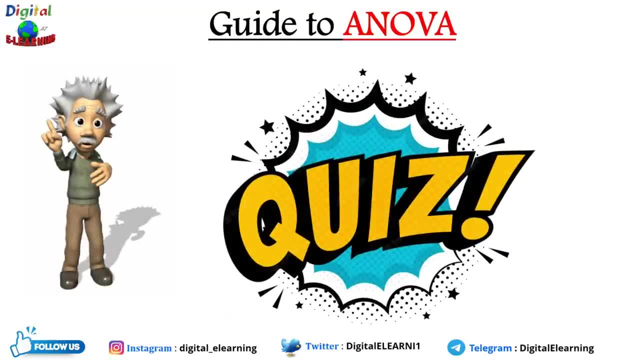 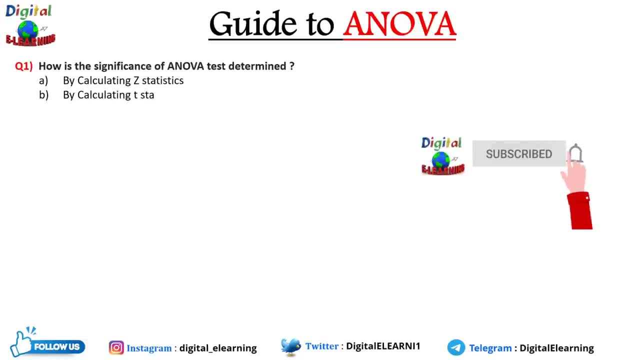 and hence the H naught is not true. that is one way ANOVA table for you. so if you are still watching this video, let's have a quick quiz. so first question: how is the significance of ANOVA test determined? by calculating Z statistics, by calculating the